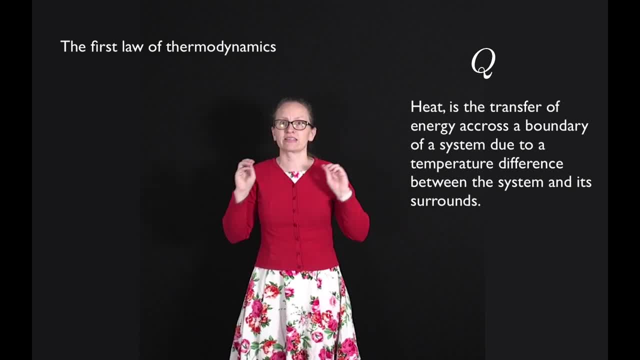 the letter capital Q and it's defined as the transfer of energy across a boundary of a system due to a temperature difference between the system and its surrounds. So heat is always transferred from the body at the higher temperature to the body at lower temperature. Now, because it's an energy transfer, it's got the same units as energy, So the units for heat. 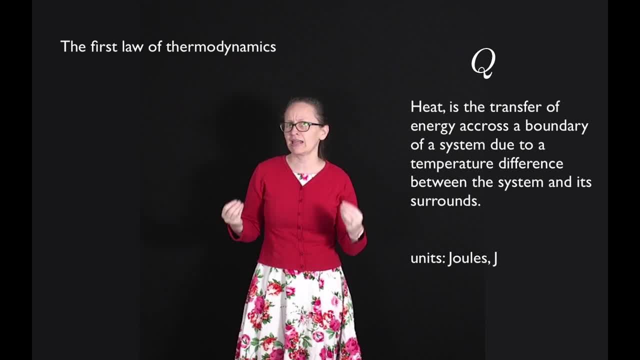 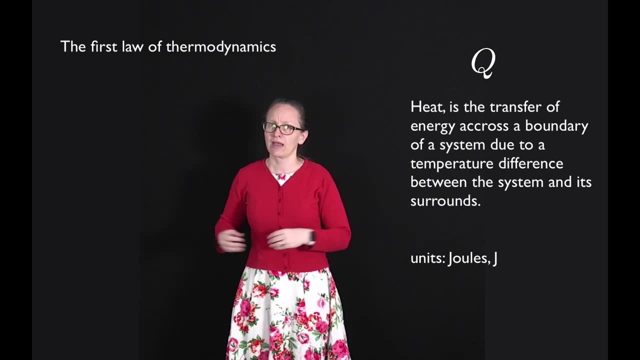 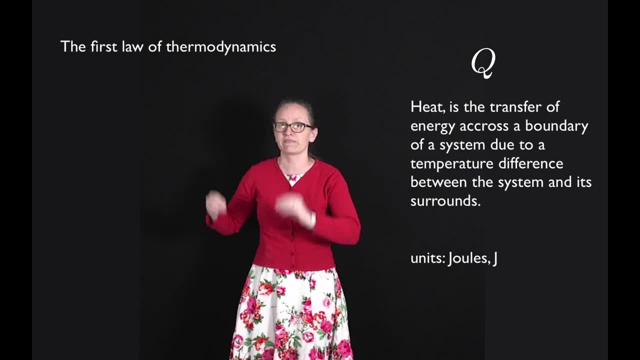 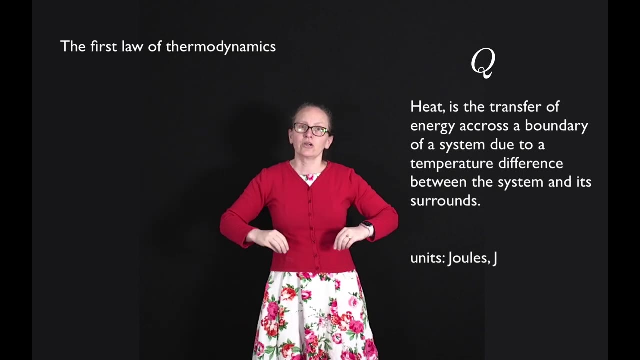 by heat in that statement. what we mean by heat formally in this course, As heat is a way of transferring energy, it's not the storage of energy in the system. So just be a little bit careful about how you interpret heat. So in the mechanics part of this course we saw that. 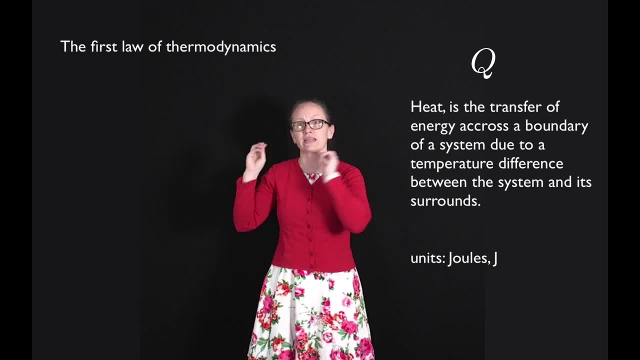 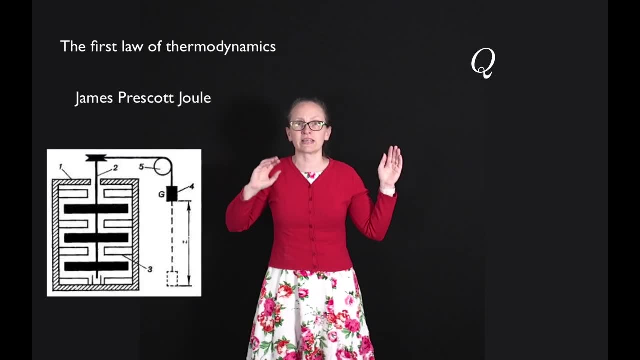 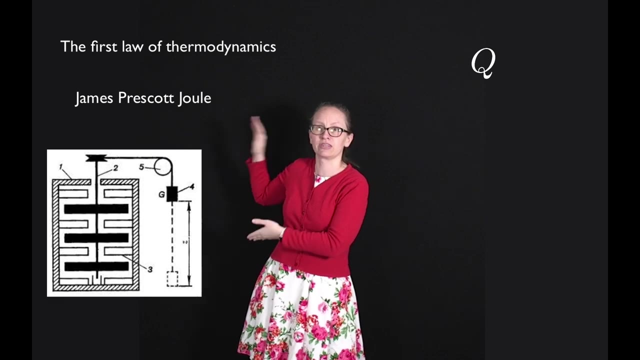 another way to transfer energy from one system to another was to do work on the system. So James Prescott Joule actually did a lot of experiments with doing work on water with a setup similar to this one between 1844 and 1854. What he found was that if he had a mass which 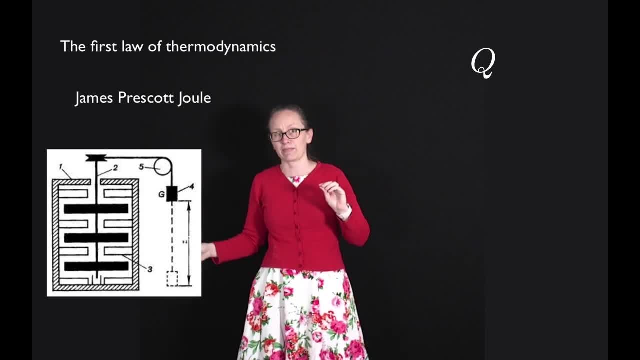 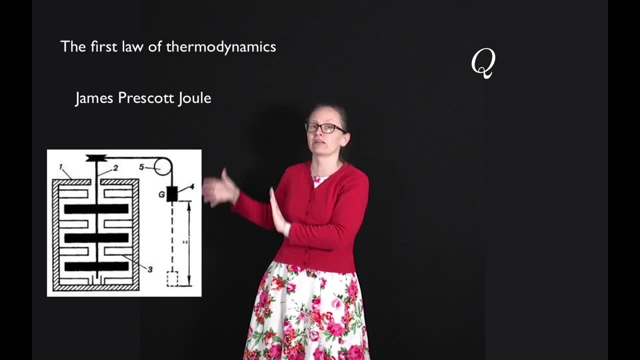 was dropping under the influence of gravity, so the hanging mass was losing gravitational potential energy. he could get this to turn paddle wheels inside a calorimeter which contained water And as the mass dropped there was a slight temperature change of the calorimeter and the 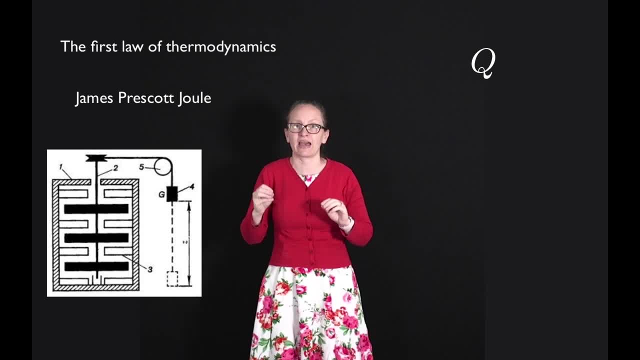 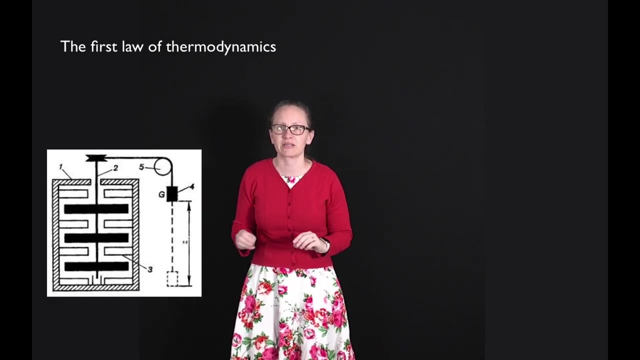 water inside it and from this he could see that the amount of work done on the water inside the system was proportional to the heat that was transferred. So this brings us to the first law of thermodynamics. The first law of thermodynamics tells us that the change in internal energy of the 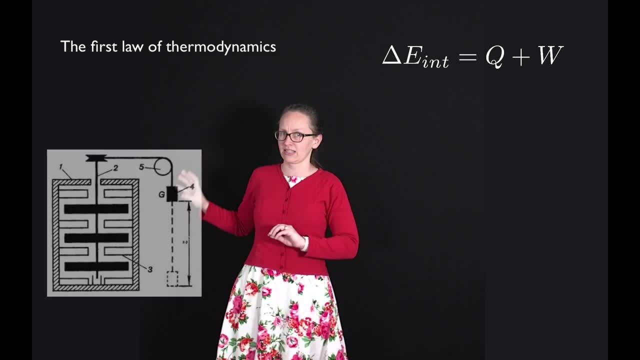 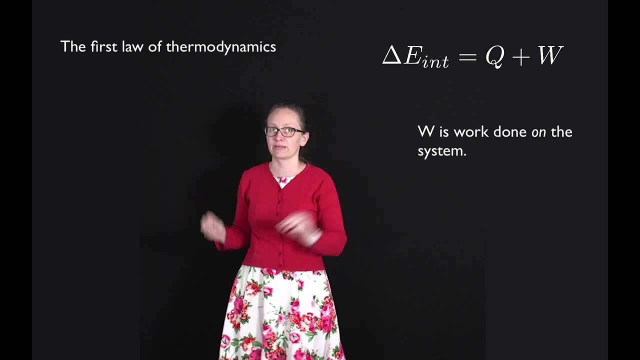 is equal to the heat transferred to the system plus the work done on the system. Now notice that I said work done on the system. In some textbooks they define W as the work done by the system, in which case it has the opposite sign. 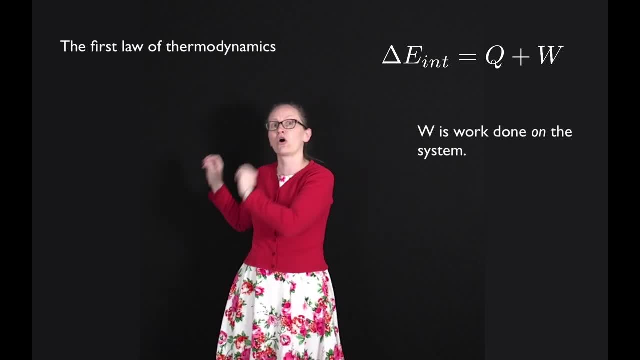 But in this course we'll use W to mean the work done on a system. So, in order to work out how to calculate this, let's consider a syringe. So here I have a syringe filled with gas. Now we know from mechanics that the amount of work done on a system is equal to the force. 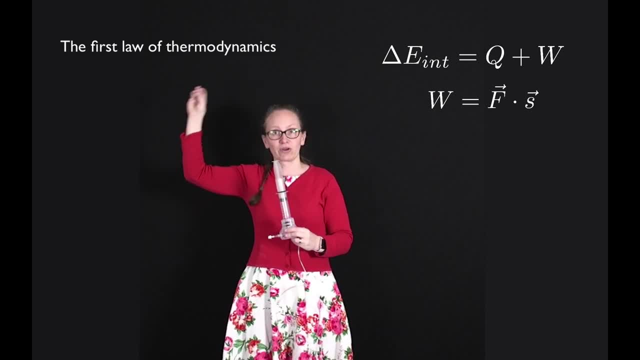 times the displacement, And by times there I mean taking the dot product. So if I apply a force onto gas in a cylinder like this, then I am doing work on the gas. So let's calculate how much work. Let's consider moving the piston down just a small height. 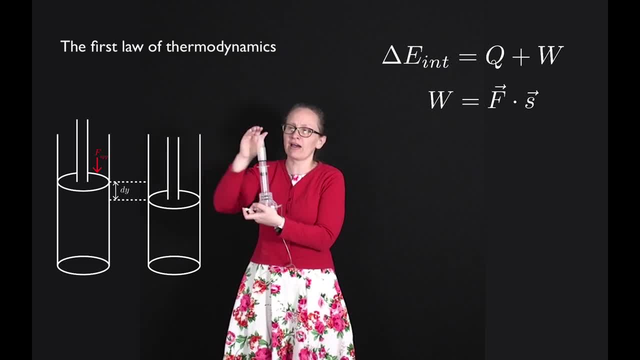 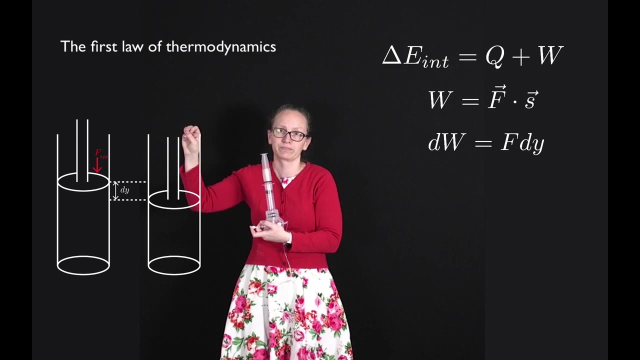 And let's call the height difference dy. So if I apply some force and the piston moves down a distance, dy, then I'm applying the force in the same direction as the displacement, And so I've got dw is equal to f dy. Now we've learned about the pressure of a gas before and we've seen that it's related. 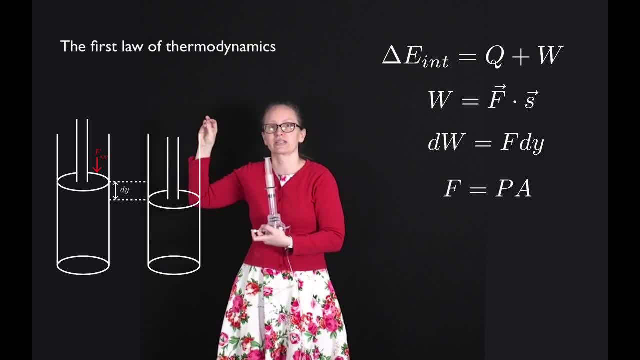 to the force through. force is equal to pressure times area. So the molecules of gas inside my syringe are applying a distance dy. So if I apply some force and the piston moves down a distance dy, then I'm applying the force in the same direction as the displacement. 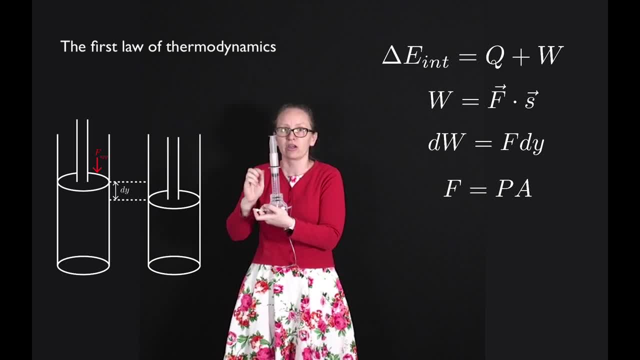 So I'm applying a force upwards on the syringe, So they're applying a force upwards and equal to pa. So if I think about the relationship between the force that I'm applying and the force that the gas molecules are applying whenever it's in equilibrium, then these two forces 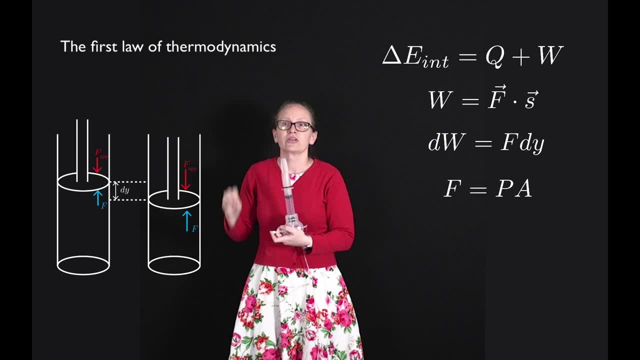 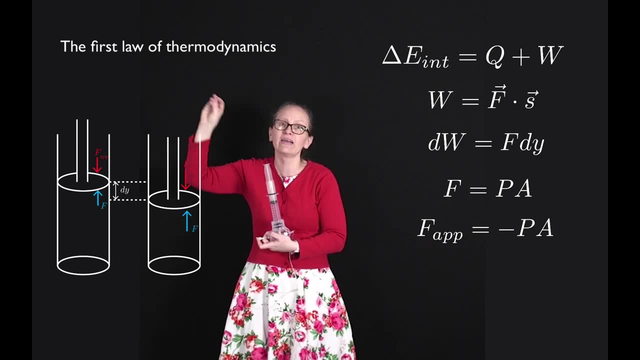 are equal. They are in opposite directions though, So I can say that f, where f stands here for the applied force, is equal to minus pa, where p is the pressure, The pressure of the gas, and a is the cross-sectional area of my syringe. 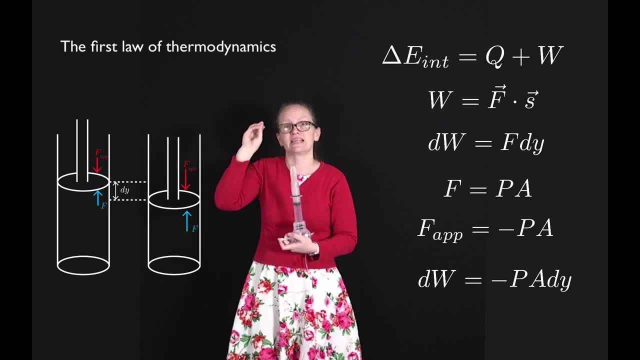 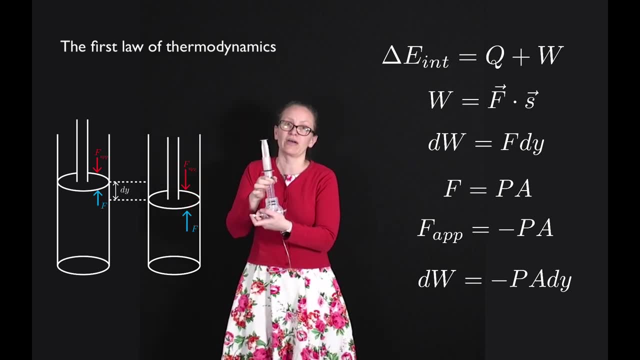 So, going back to my equation for dw, I've then got that dw is equal to minus pa dy And a times dy. well, that's the cross-sectional area times the change in height, which is just the change in volume of my gas.